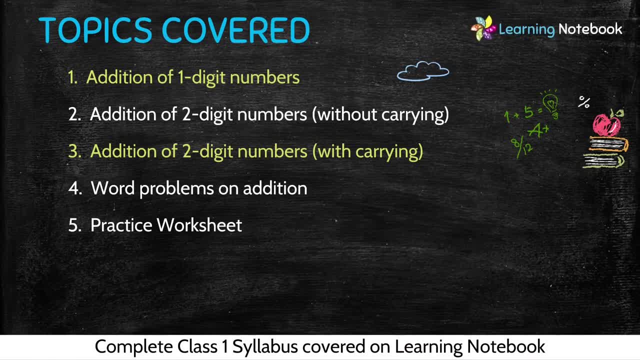 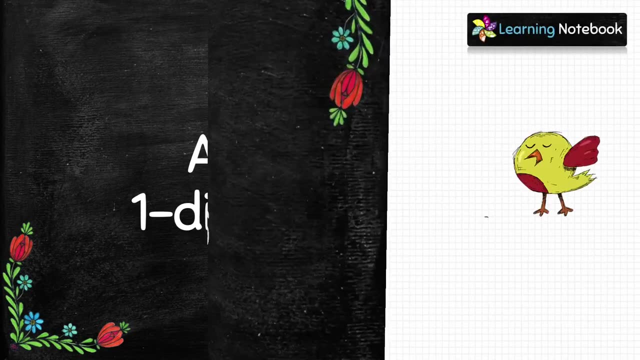 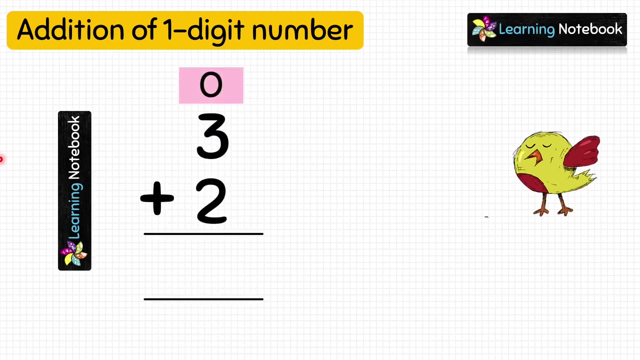 After that we will solve word problems related to addition And in the end, students, I will give you a worksheet for your practice. So let's start with addition of one digit numbers. Let's see how to add 3 and 2 vertically. We will represent. 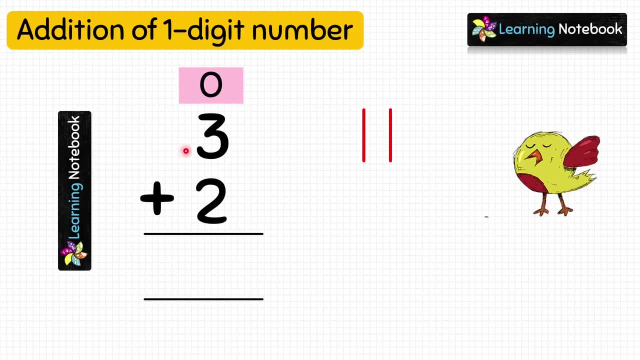 3 as 3 lines. So draw 3 lines. and similarly represent 2 as 2 lines. So let's draw 2 lines here, Then we will count all these lines. So let's count them: 1, 2, 3, 4,, 5, 6, 7,. 8,, 9,, 10,, 11,, 12,, 13,, 14,, 15,, 16,, 17,, 18,, 19,, 20,, 21,, 22,, 23,, 24,, 25,, 26,, 27,, 28,, 29,, 30,. 30,, 31,, 32,, 33,, 34,, 35,, 36,, 37,, 38,, 39,, 40,, 41,, 42,, 43,, 44,, 45,, 46,, 47,, 48,, 49,, 50,, 51,. 52,, 52,, 53,, 42,, 45,, 47,, 58,, 51,, 52,, 53,, 52,, 54,, 57,, 58,, 51,, 52,, 53,, 53,, 52,, 53,, 52,, 53,, 53,, 53,. 52,, 53,, 54,, 57,, 52,, 53,, 53,, 53,, 53,, 53,, 54,, 57,, 58,, 57,, 58,, 58,, 59,, 59,. 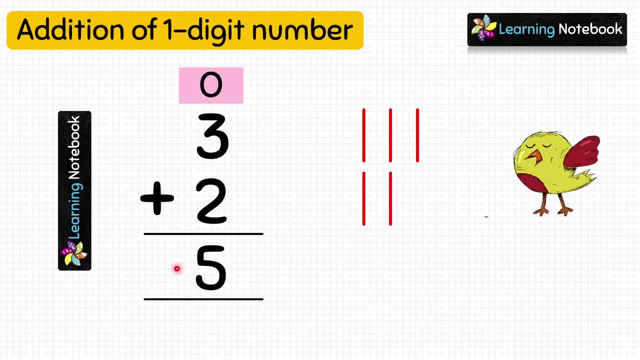 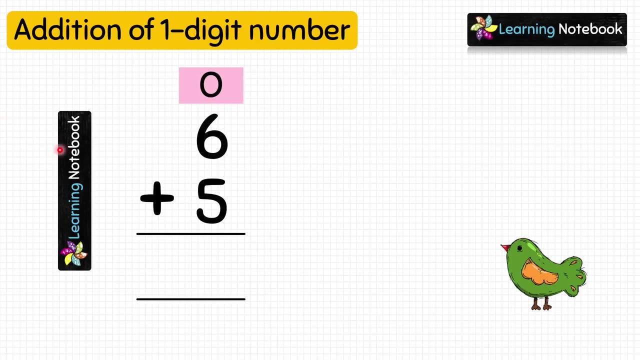 So answer is 5.. It means 3 plus 2 equals to 5.. Now let's add 6 and 5 vertically, So we will represent 6 as 6 lines. So let's draw 6 lines here, Then we will represent 5 as. 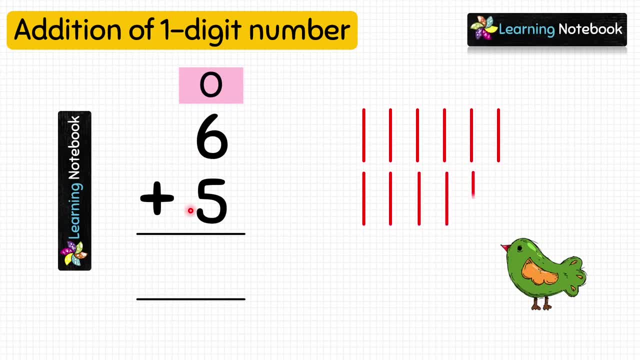 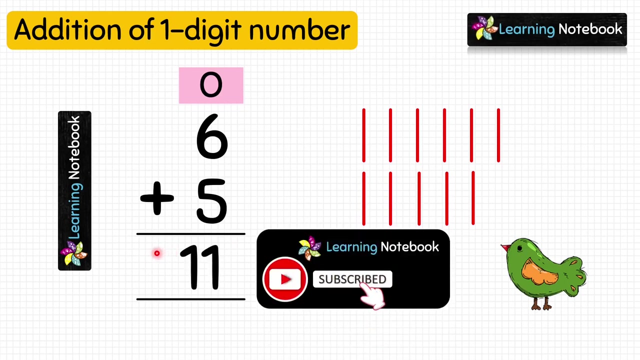 5 lines. Now, students, we will count all these lines: 1,, 2,, 3,, 4,, 5, 6,, 7,, 8,, 9,, 10, 11.. So 6 plus 5 equals to 11.. If you still not have subscribed to our 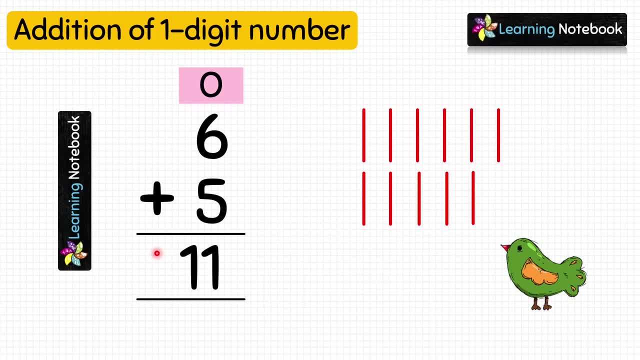 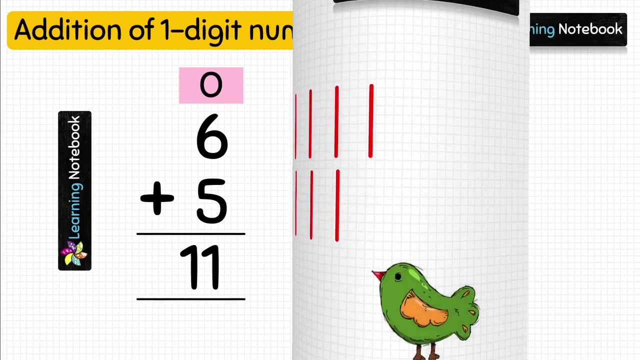 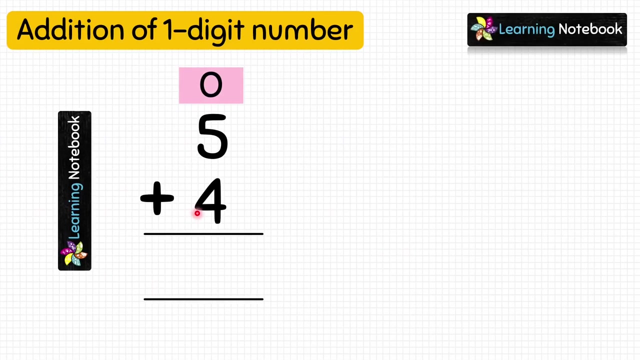 channel Learning Notebook, then do subscribe it and make sure to press the bell icon. So, students, this was one way to add numbers. Now let me tell you another way to add these numbers. For example, we have to add 5 and 4.. So to add them, we will first keep the bigger number. 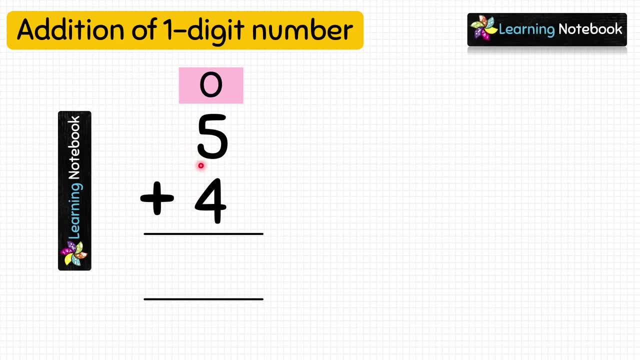 in our mind Here, bigger number is 5.. So let's keep 5 in our mind And count 4 on our fingers. So after 5, count on fingers 6,, 7,, 8,, 9.. So 9 is our answer. 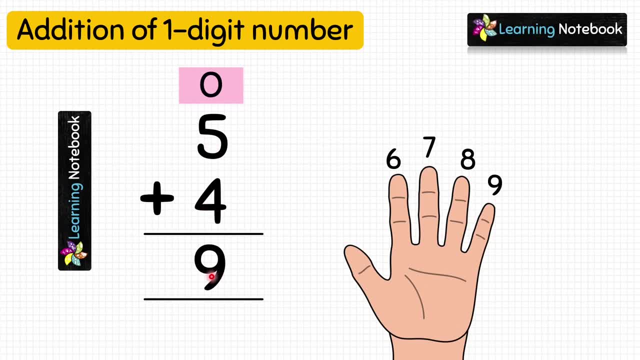 5 plus 4 equals to 9.. Let me tell you this method once again. So to add these numbers: first we will keep the bigger number, that is 5, in our mind, Then we will count 4 on our fingers. So after 5, let's count on fingers 6,, 7,, 8,, 9.. So 9 is our answer. 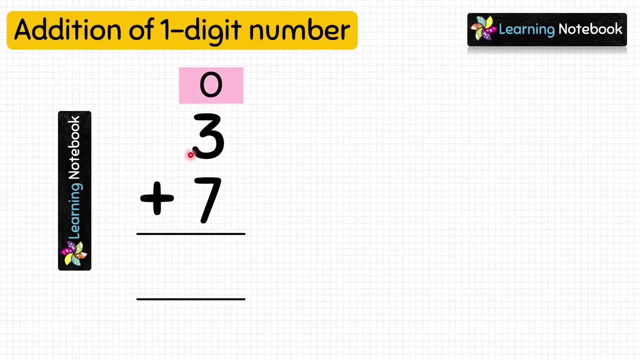 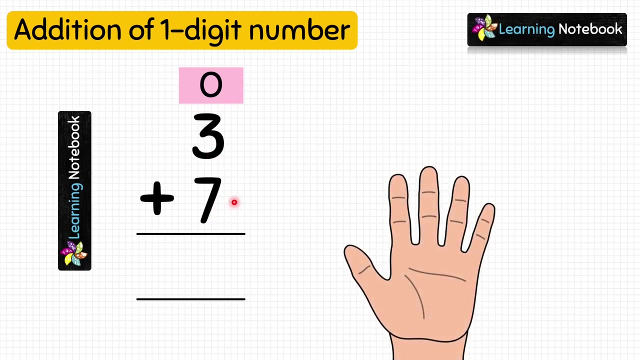 Next question is: add 3 and 7.. So here, which one is the bigger number? Yes, 7.. So let's keep 7 in our mind And count 3 on our fingers. So after 7, count 3 fingers. 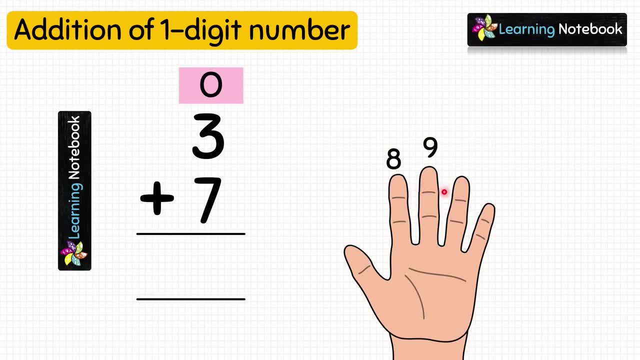 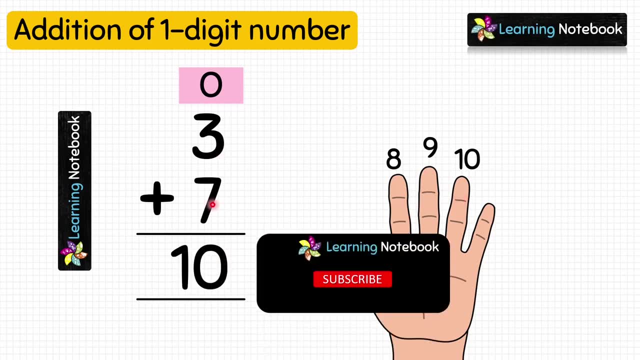 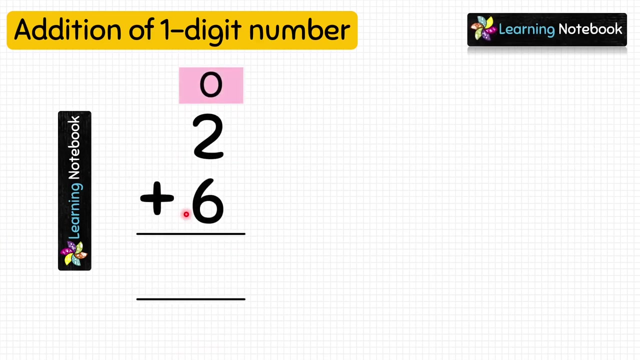 8,, 9,, 10.. So this is our answer: 10. 3 plus 7 equals to 10.. Let's do one more example: Add 2 and 6.. So to add them, keep the bigger number. 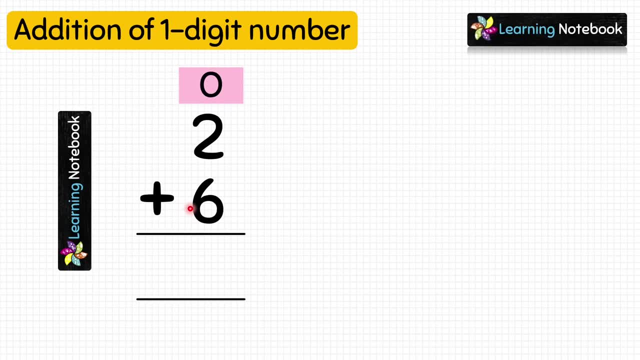 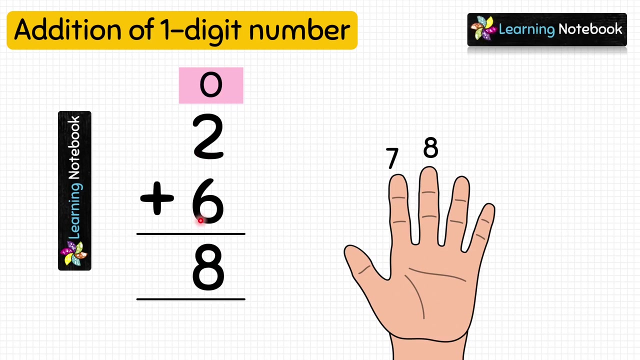 Keep the bigger number in mind, which is 6. And add 2 to it. How will we add 2 to it? We will count 2 fingers after 6.. So count 7, 8.. So this is our answer: 8.. So 2 plus 6 equals to 8.. 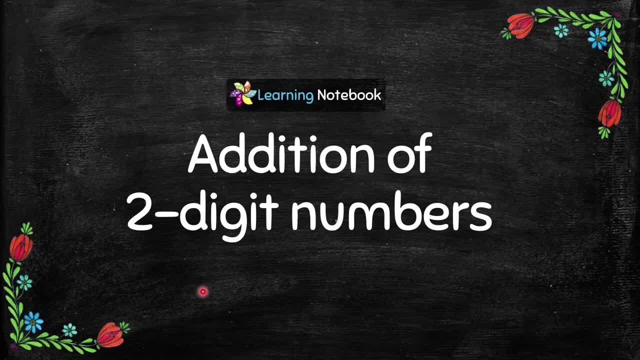 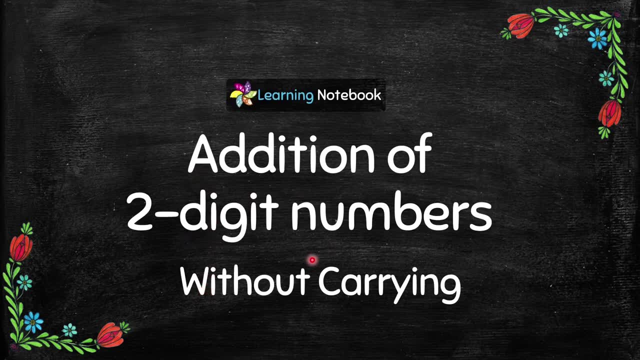 So, students, now I am going to tell you another method. So let's do one more example, And I am sure you have understood this second way to add numbers. Now let's do addition of 2-digit numbers without caring. 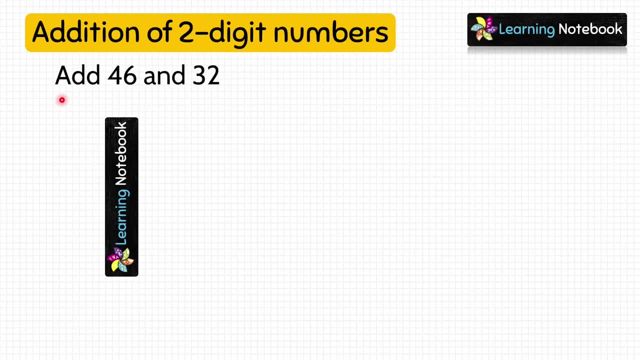 So now, students, we have to add 2-digit numbers. Numbers are 46 and 32.. First of all, write them as shown here, That is, digits at 1's place under 1's column and digits at 10's place under 10's column. 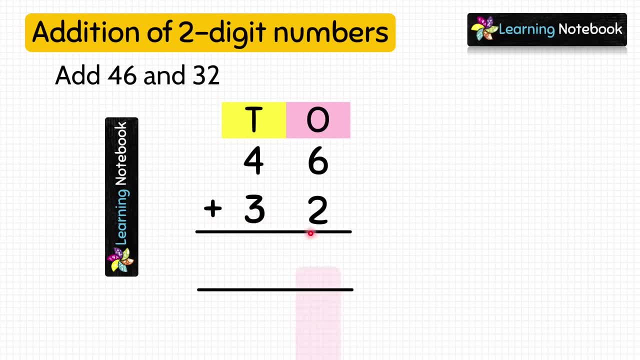 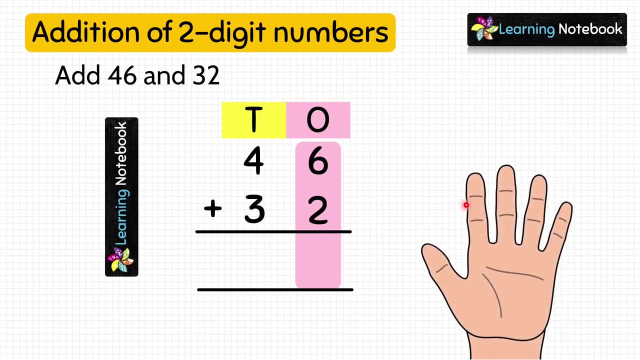 Now to add them. first we will add the digits at 1's place, which are 6 and 2.. So add them in the same way as we did earlier. We will keep the bigger number, Number 6, in mind and count 2 on fingers. 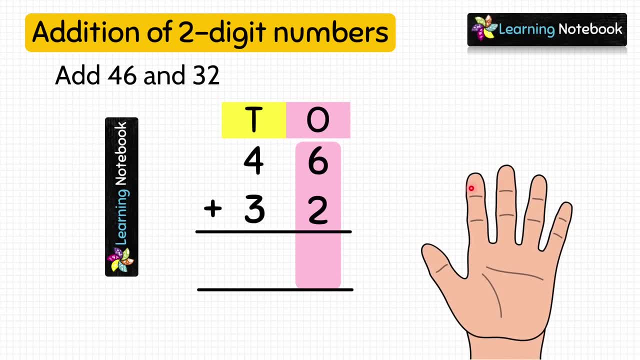 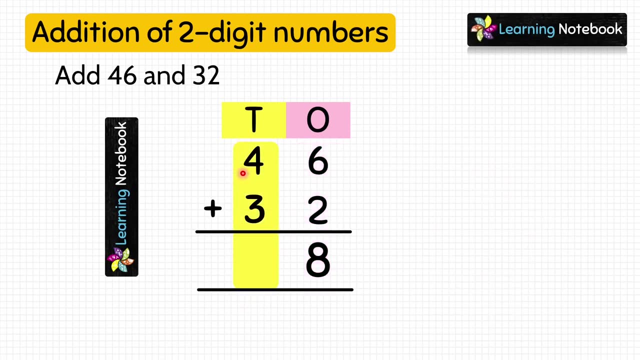 So after 6, count 2 fingers, 7,, 8.. So write 8 here. Now add digits at 10's place Again, which is the bigger number here out of 4 and 3? 8.? 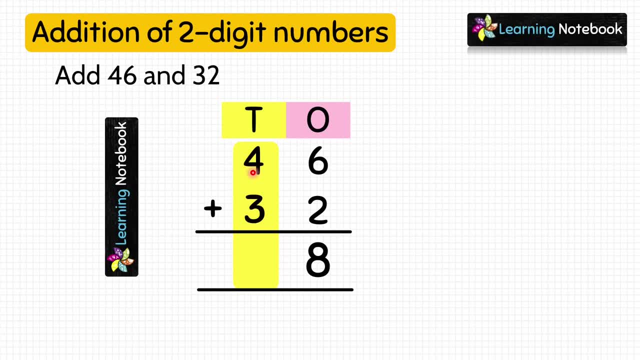 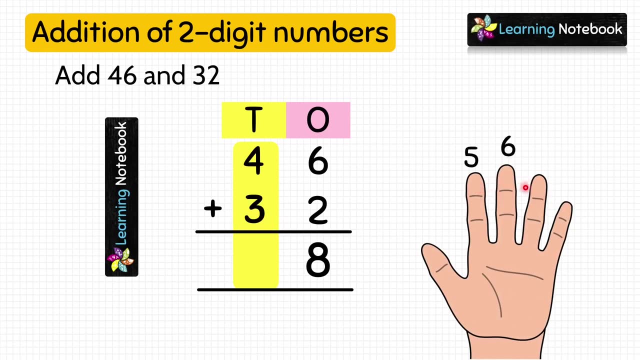 Yes, 4 is the bigger number. So keep 4 in your mind and count 3 on fingers. So, after 4, count 3 fingers, 5,, 6, 7.. Write 7 here, So our answer is 78.. 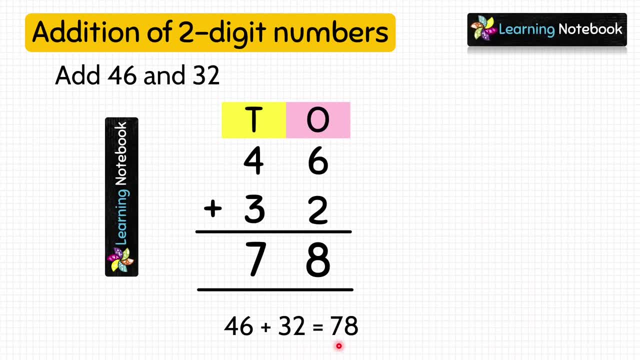 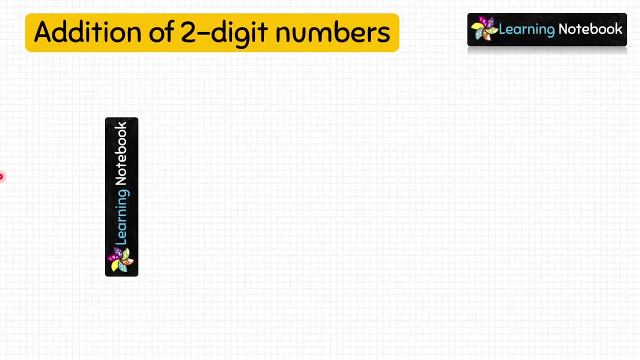 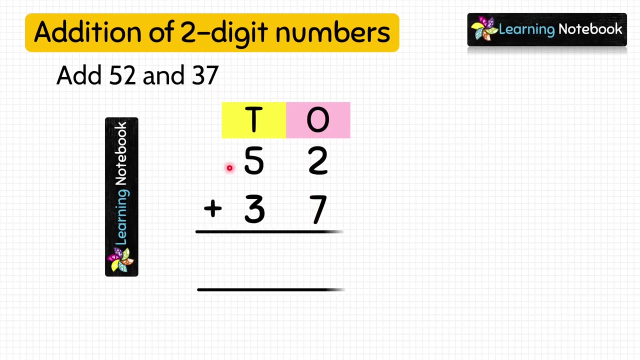 8.. 46 plus 32 equals to 78.. Let's do one more question: Add 52 and 37. So to add these two 2-digit numbers first, we will write them in column form. It means digits at 1's place under 1's column and digits at 10's place under 10's column. 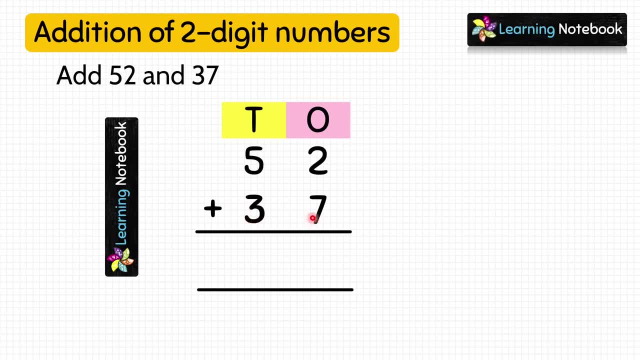 So we will write them in column form. It means digits at 1's place under 1's column and digits at 10's place under 10's column. Now, first we will add the digits at 1's place, We will keep bigger number in mind, which is 7, and then count 2 fingers. 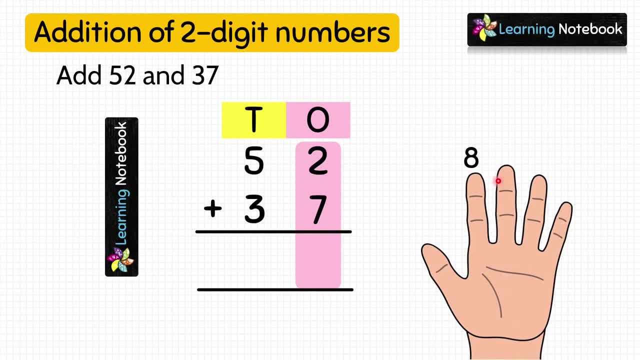 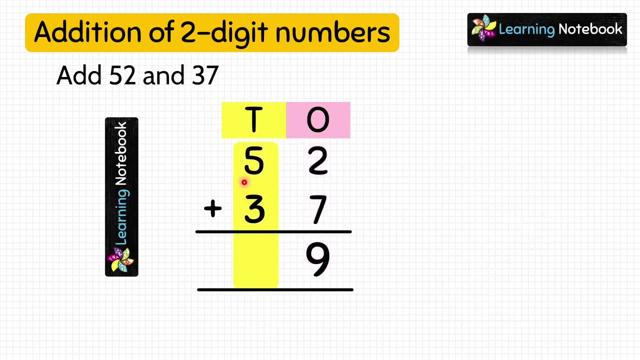 So after 7, count 2 fingers, 8,, 9.. So write 9 here. Now let's add the digits at 10's place, Let's keep bigger number 5 in our mind and count 3 fingers. 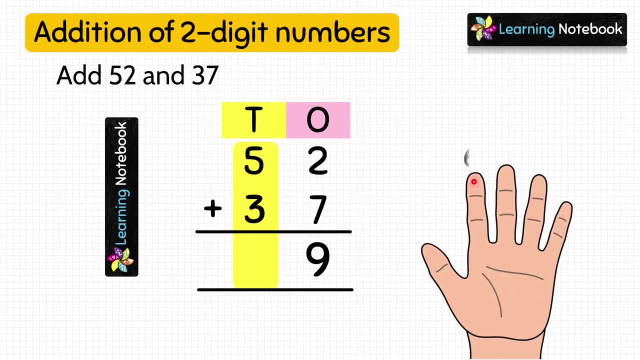 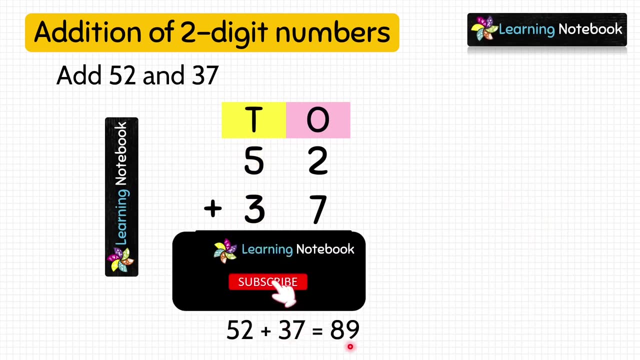 So after 5, let's count 3 fingers: 6,, 7,, 8.. So write 8 here. So this is our answer: 89, 52 plus 37 equals to 89.. 89.. 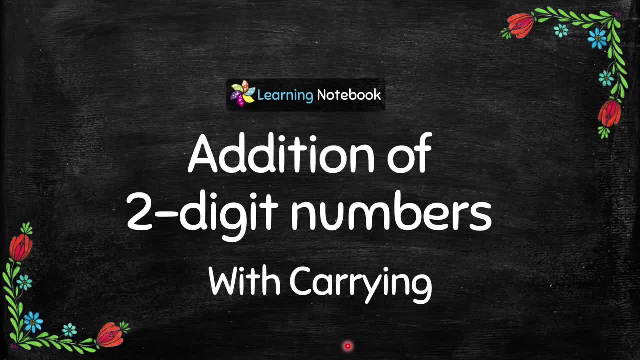 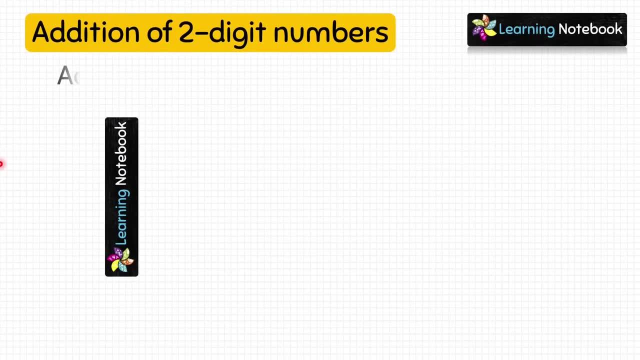 Now, students, we will learn how to do addition of 2 digit numbers with carrying Question is add 46 and 14.. So to add these 2 numbers first, we will write them in column As shown. Now. let's add the digits at one's place. 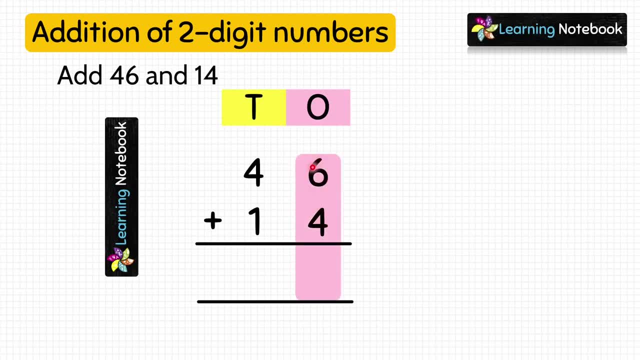 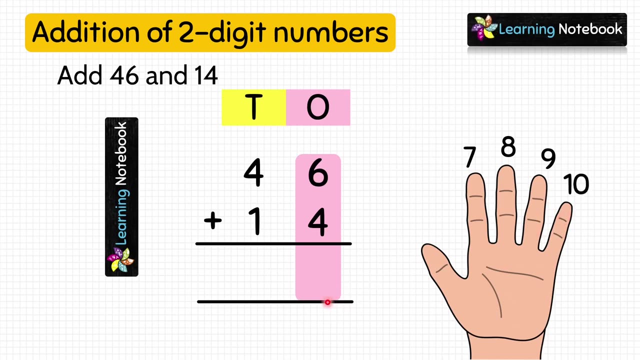 So let's keep bigger number 6 in mind and count 4 on fingers. So after 6, count 4 fingers, 7,, 8,, 9,, 10.. So we have got 10.. Now students in 10.. 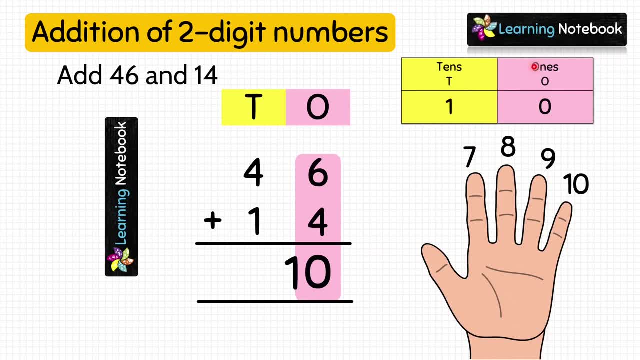 0 is at 1's place and 1 is at 10's place. So in the answer 0 will remain at 1's place, But 1 will go at 10's place. So let's carry 1 to the 10's place. 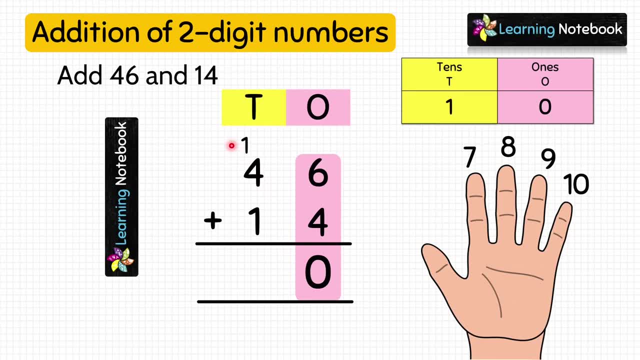 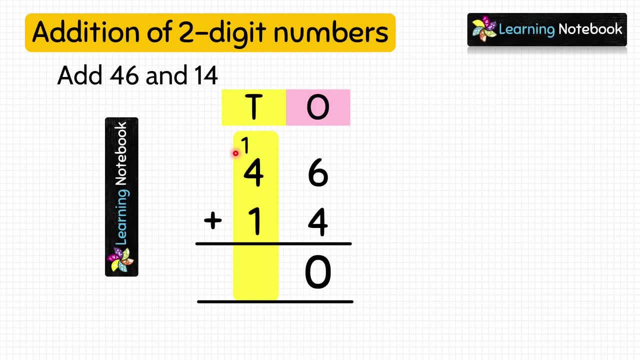 Now let's add the digits at 10's place Here. students, now you have to make sure that you add this: carry 1 to the digits at 10's place. So now we have 3 numbers to add here. 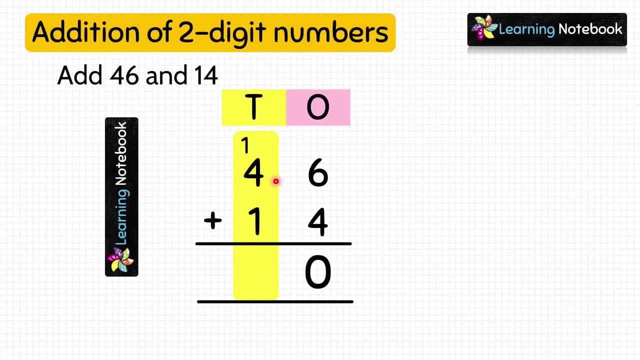 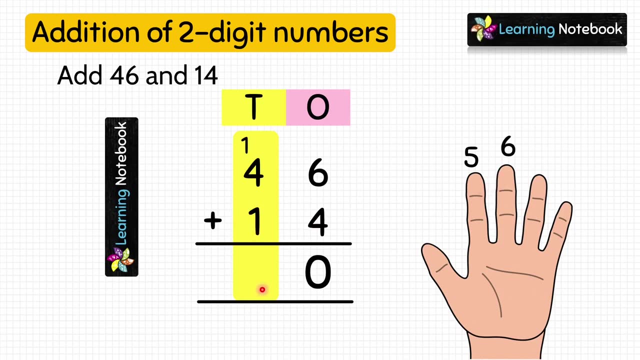 So let's keep bigger number 4 in mind. Then count 1 finger, We get 5.. And then count 1 more finger, We get 6.. So write 6 here. So we have got the answer as 60.. 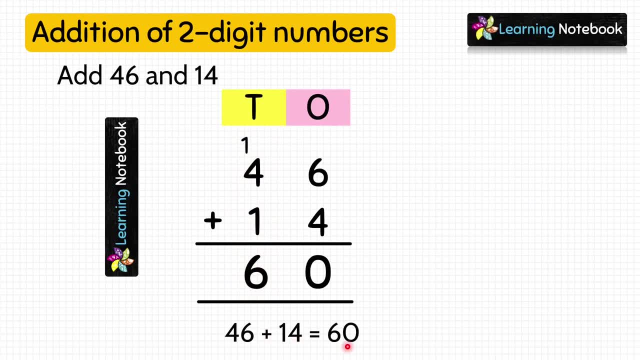 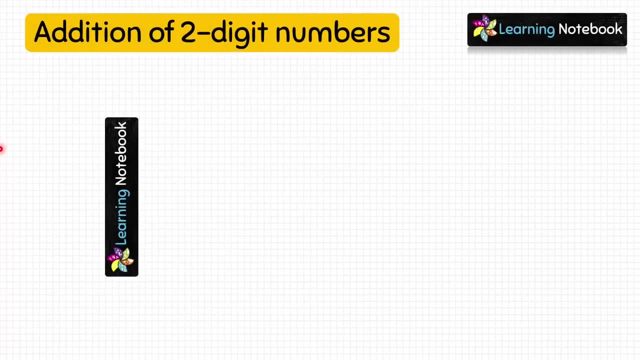 46 plus 14 equals to 60. So, students, this is how we do addition of 2 digit numbers with carrying. Let's do one more question. Question is: add 64 and 38. So first write them in column form. 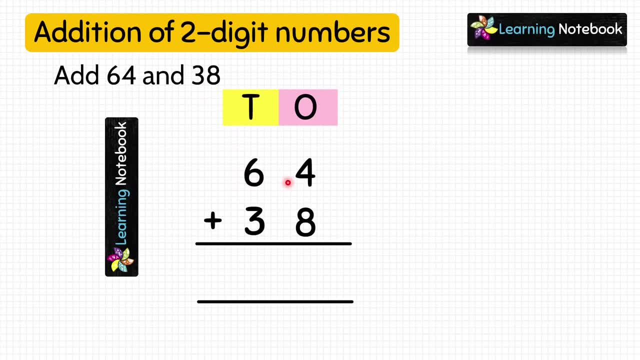 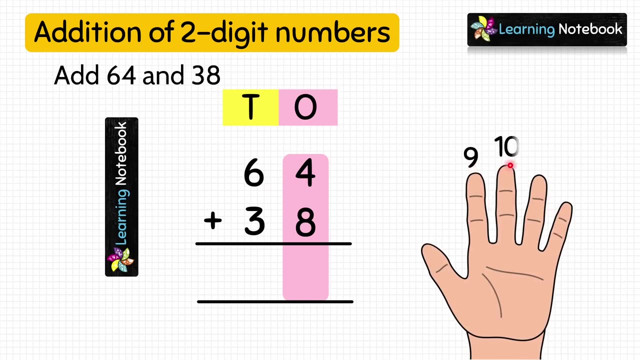 Then start adding the digits at 1's place. For this, keep bigger number 8 in your mind and count 4 fingers. So we get 9,, 10,, 11,, 12.. Now students in 12,: 2 is at 1's place and 1 is at 10's place. 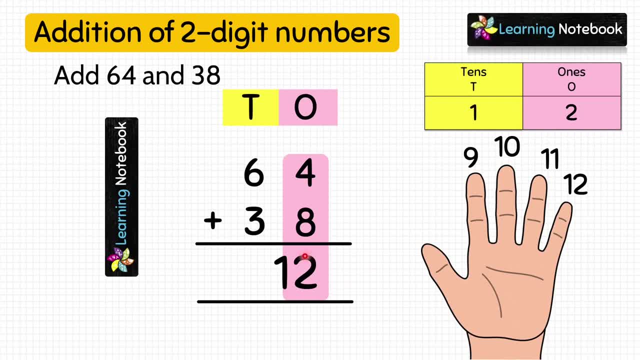 So in the answer 2 will remain at 1's place And we will carry 1 to the 10's place. So in the answer, 2 will remain at 1's place and we will carry 1 to the 10's place. 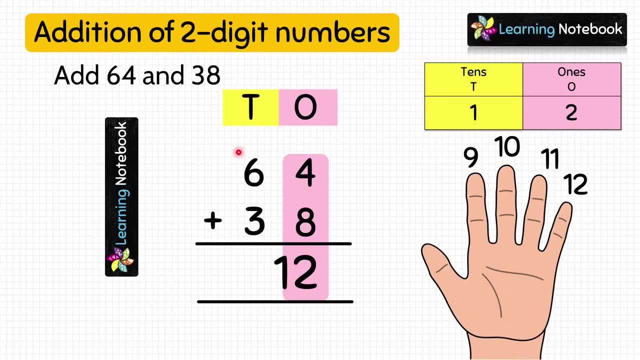 So in the answer, 2 will remain at 1's place. So in the answer, 2 will remain at 1's place and we will carry 1 to the 10's place. Right Now, let's add the digits at 10's place. 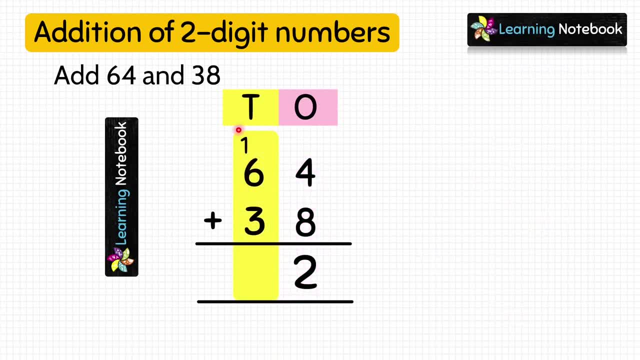 Just make sure that you add this carry 1 to the digits at 10's place. So now we have to add 3 numbers here. So keep bigger number 6 in your mind. So now we have to add 3 numbers here. 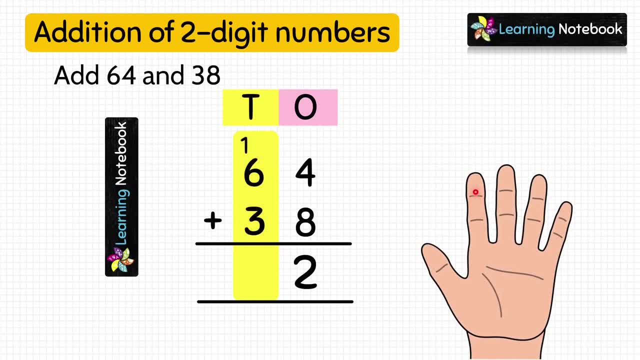 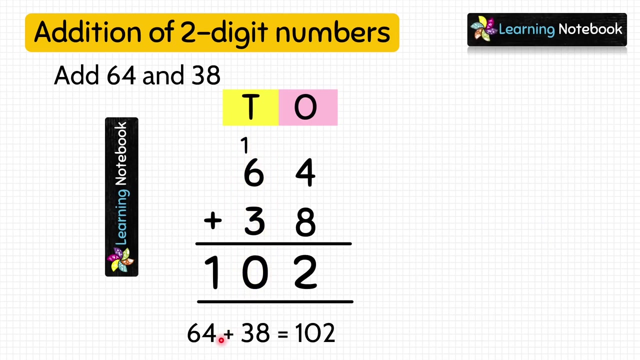 And count 1 finger, We get 7.. Now count 3 fingers: 8,, 9,, 10.. So we will write 10 here. This is our answer: 102.. 64 plus 38 equals to 102.. 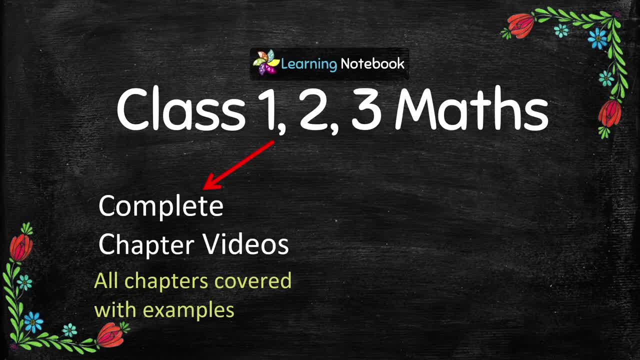 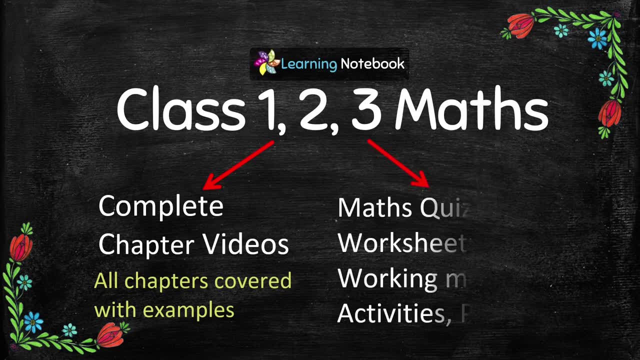 Students. we would like to tell you that we have made videos on every chapter of Class 1,, Class 2 and Class 3 Mathematics. We also have interesting Maths quizzes, Worksheets, Test Papers, Working Models, Activities and Projects on each chapter. 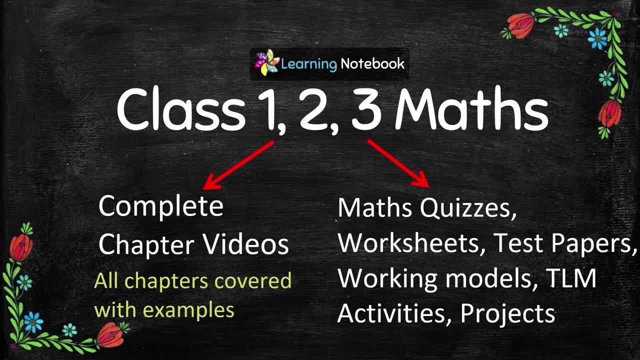 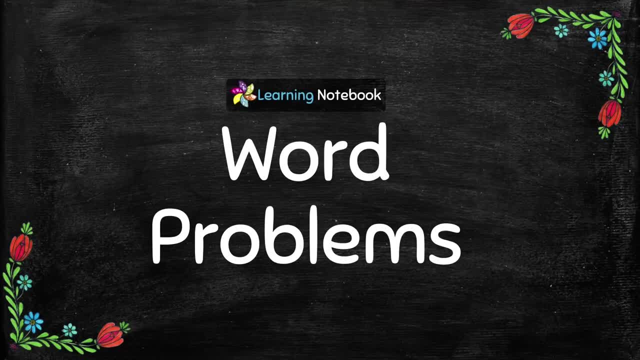 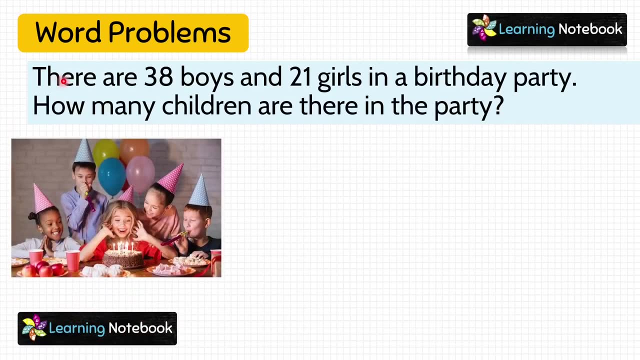 So I would suggest you to check out our channel Learning Notebook. Now let's solve word problems related to addition. Question is: there are 38 boys and 21 girls in a birthday party. How many children are there in the party? So here we are given: number of boys and number of girls in a birthday party. 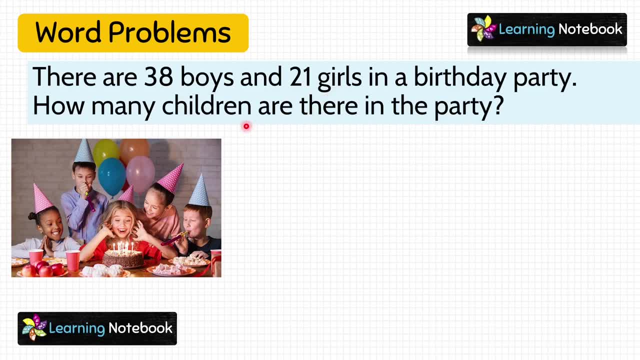 And we have to find total children in that party. So to find this, we will add 38 and 21. So let's add them First. we will write them in column form. Now start. Start adding the digits at 1's place. 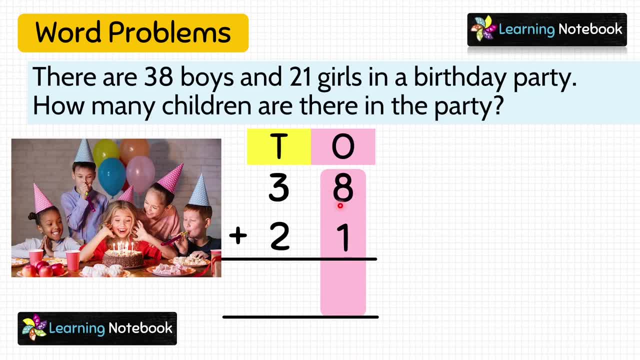 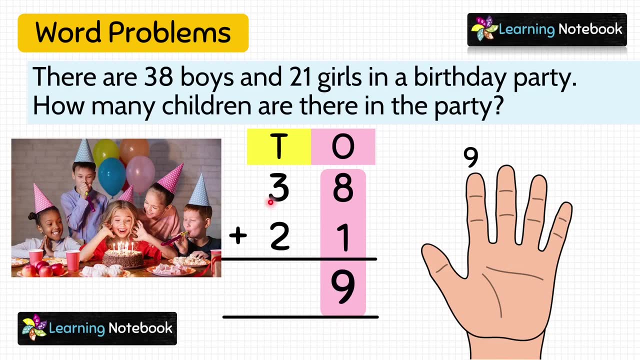 So keep bigger number 8 in your mind and count 1 finger, So we get 9.. We will write 9 here, Then add the digits at 10's place. Keep bigger number 3 in your mind And count 2 fingers. 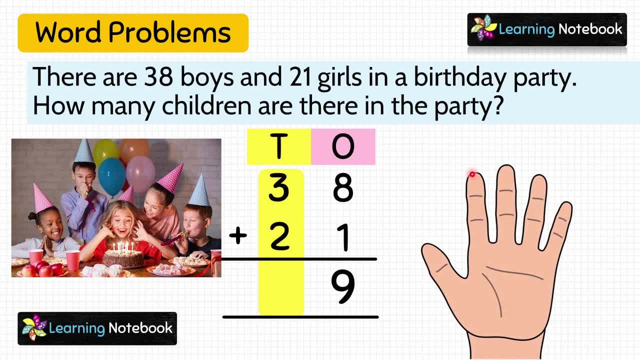 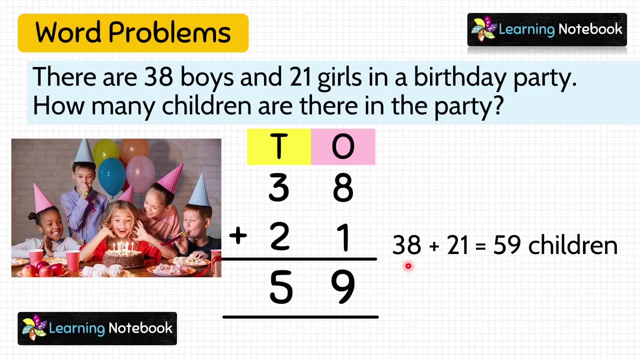 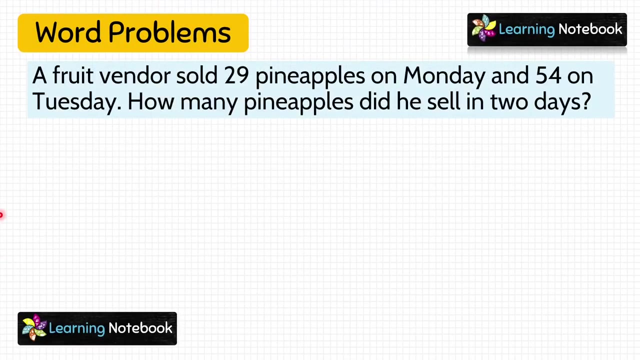 So after 3, count 2, fingers, 4,, 5. Write 5 here. So we have got the answer as 59.. There were 59 children in the party. Now let's do one more word. problem: A fruit vendor sold 29 pineapples on Monday and 54 pineapples on Tuesday. 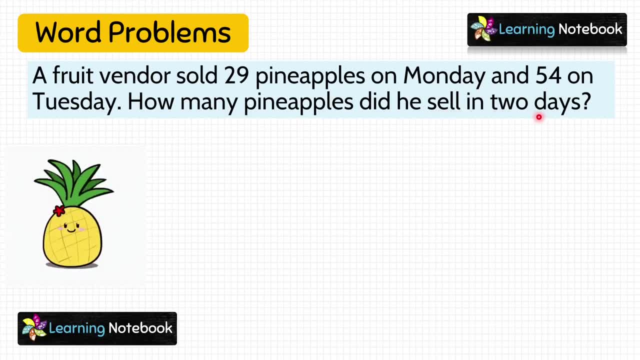 How many pineapples did he sell in 2 days? So here, students, we are given with number of pineapples sold on Monday and number of pineapples sold on Tuesday, And we have to find total number of pineapples sold on Monday. 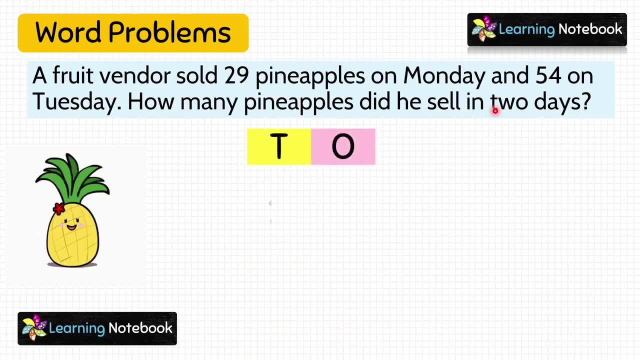 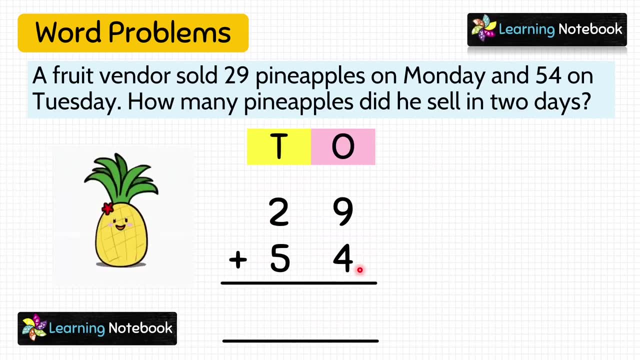 Both these days. So to find it, we will add 29 and 54. So, after writing them in column form, let's add the digits at 1's place. Keep bigger number 9 in your mind and add 4 fingers. 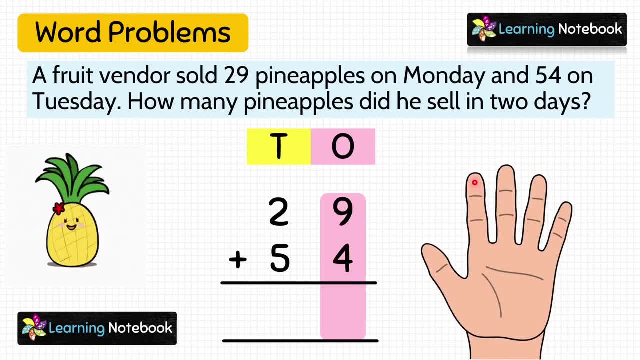 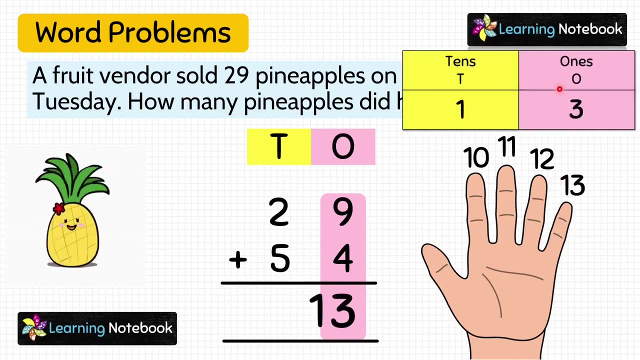 So count after 9., 10., 11., 11,, 12,, 13.. Now in 13,, 3 is at 1's place and 1 is at 10's place. So 3 will remain at 1's place in the answer and 1 will go to 10's place. 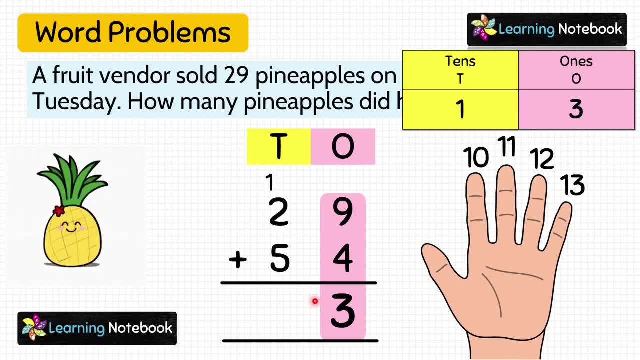 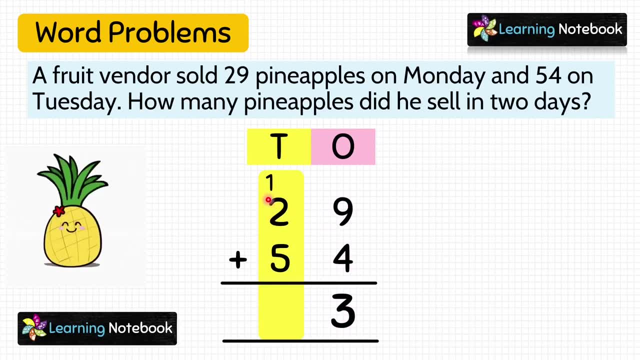 So let's carry 1 to the 10's place. Now. let's add the digits at 10's place Now. here we will add this: carry 1 also. So let's add 3 digits here. Keep bigger number 5 in your mind and count 2 fingers. 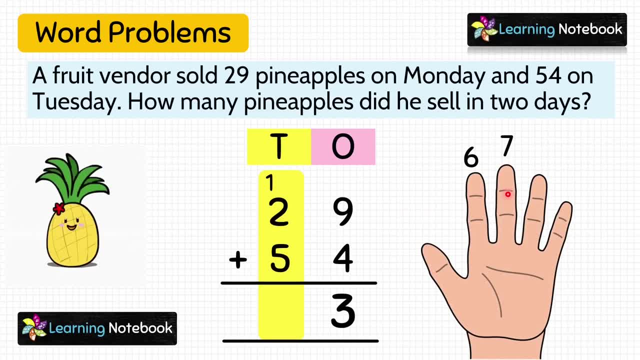 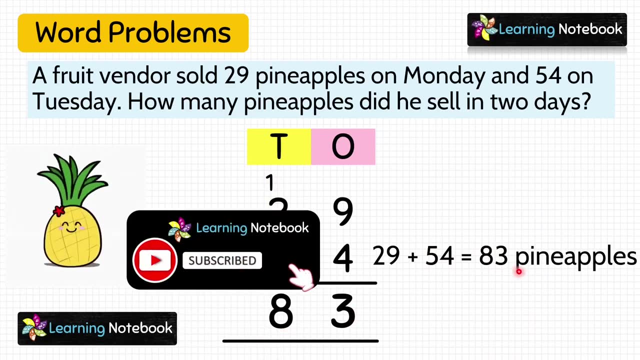 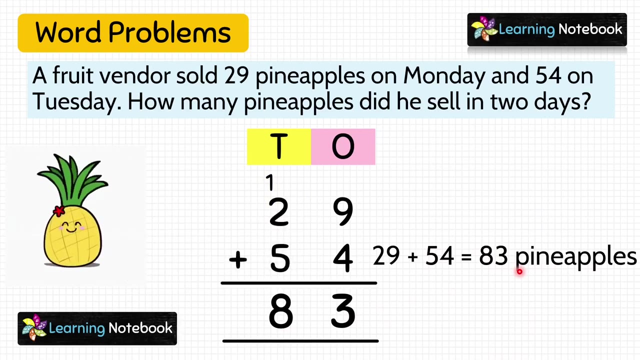 6, 7.. Now count 1.. One more finger, We get 8.. So write 8 here. This is our answer: 83.. 83 pineapples were sold in 2 days. So, students, now I am sure you have understood how to do addition of 1 digit number.